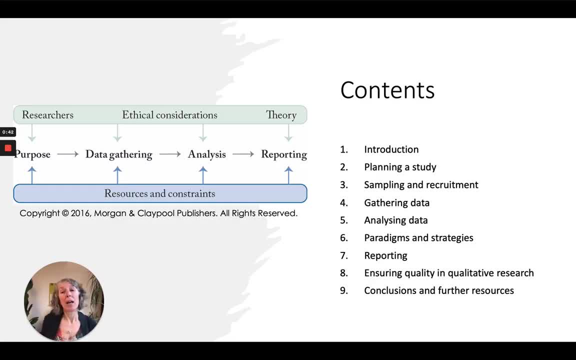 reporting a qualitative study involving all the steps from considering what the point of a study is, what's its purpose, through the key steps of data gathering and analysis, to presenting the results, including an account of all those things that you have to take account of along the way. 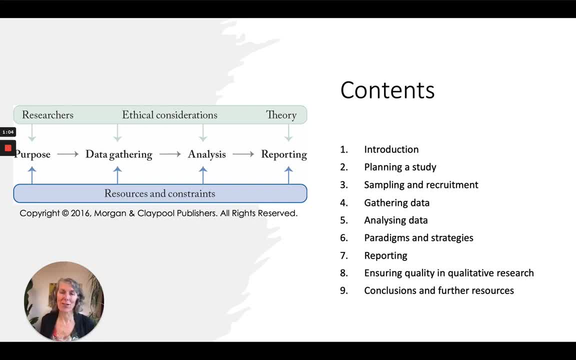 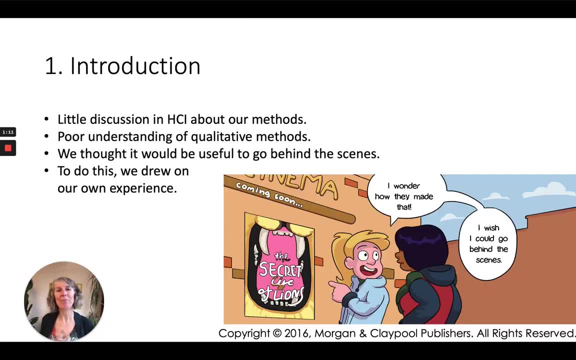 Such as your properties as a researcher, ethical concerns, any theory you might be drawing on, and resources and constraints that you're working with. Why do we write it? Well, basically, within human-computer interaction, there is little discussion about the methods that we apply, whether those are in qualitative methods, 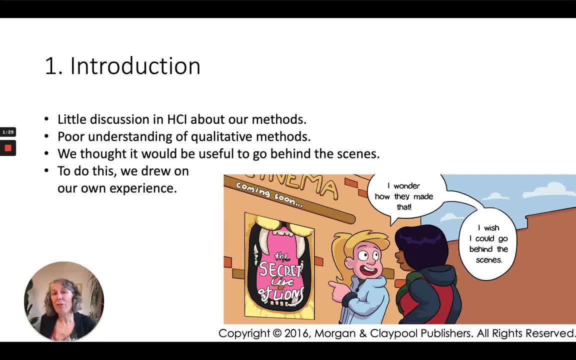 quantitative design or other forms of research. We don't talk about what we do. we draw it very often from other disciplines and I've come across many instances where people clearly have a poor understanding, particularly of qualitative methods. So we thought it would be useful to go behind the scenes and to do this. we 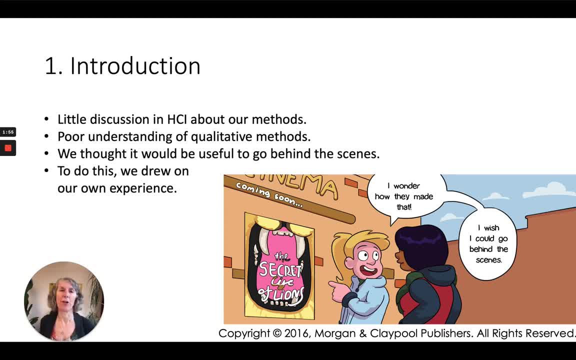 drew extensively on our own experience. But why the lions? we drew on the analogy of a wildlife film? because over several discussions between Dom Stefan and myself, we realised that there were some really nice accounts of how films had been made, particularly wildlife films where they had introduced boulder cams. 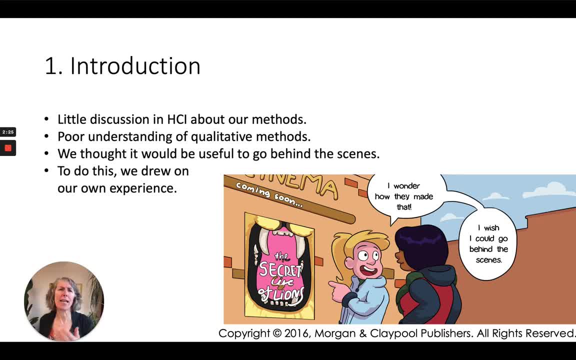 or camera crew had sat for days in freezing circumstances or very uncomfortable just to catch a shot of the target animal, or they had set up clever camera traps. so a lot of the techniques were ones that wouldn't be obvious to us as viewers, and we thought: well, something similar happens in HCI research. 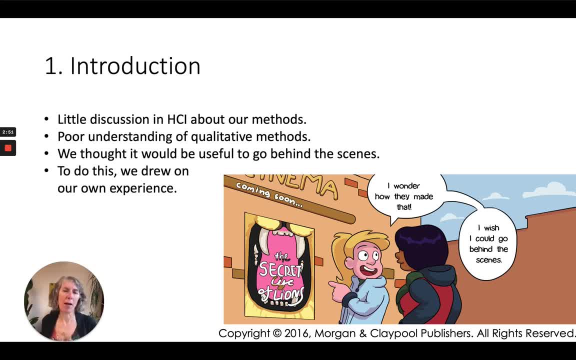 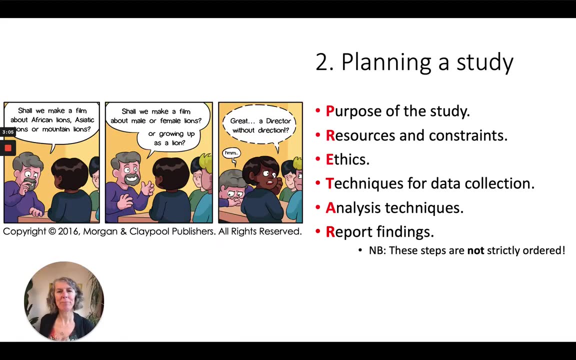 that all those details of how you go about recruitment, how you gather the data, how you do the analysis are often kind of swept under carpet when a paper is published about a study. we wanted to go behind the scenes, so we start by talking about how you plan a study. 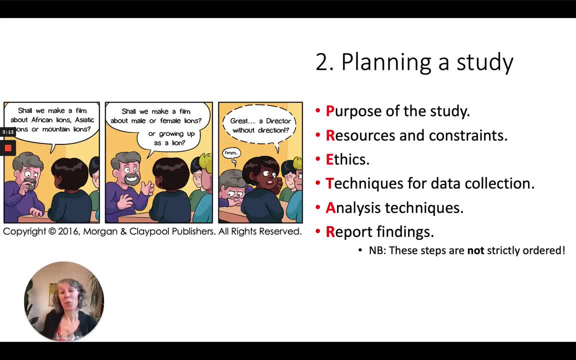 thinking about what its purpose is, what resources and constraints you're working with, and particularly ethical considerations. we talk in depth about techniques for data gathering and analysis, and then reporting and reporting findings. I've presented them in a superficially logical order here. in practice, things don't always go quite this neatly. 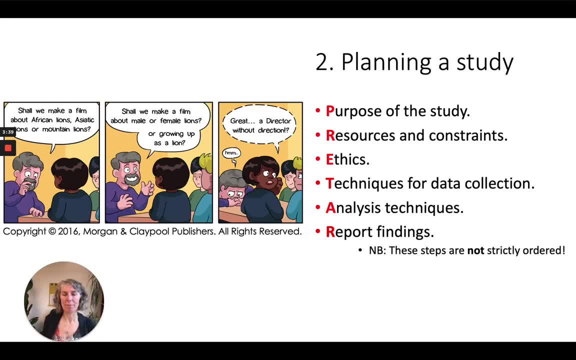 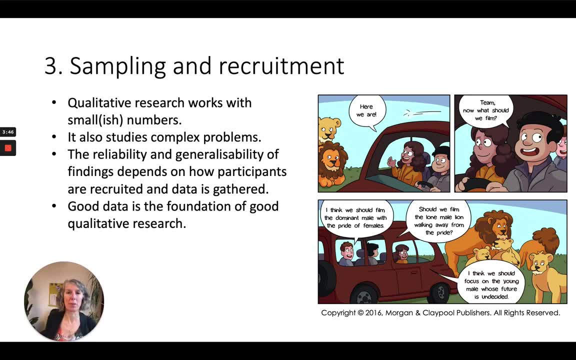 and very often there is iteration through these different steps. one key element is sampling or recruitment of participants. qualitative research works with relatively small numbers but gathers rich data. it also tends to study the data that is being collected by the participants. it also tends to study the data that is being collected by the participants. 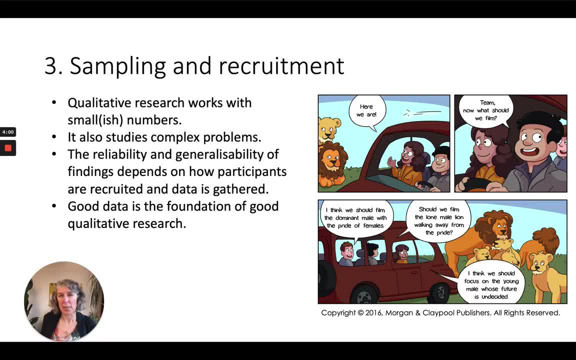 it also tends to study the data that is being collected by the participants. it also tends to study complex problems where it's not easy to decompose into simple hypotheses that can be tested. where it's not easy to decompose into simple hypotheses that can be tested. 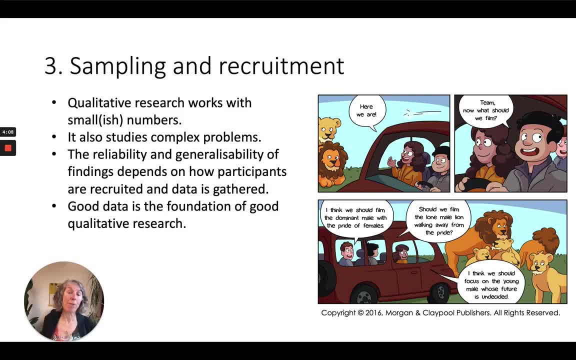 so the reliability and generalisability of findings from a qualitative study depend heavily on how participants are recruited and how the data is gathered, and good data is the foundation for good qualitative research. So it's a really important starting point and we consider it as, at some depth, 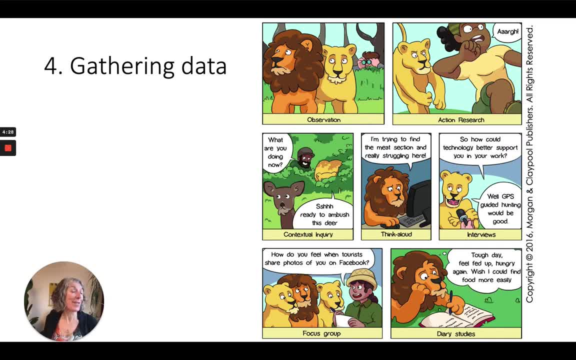 and we consider it as at some depth. The cartoon that seems to crop up most often is the one about gathering data. We cover the seven techniques that are listed here: Observation, action, research, contextual inquiry, think aloud, interviews, focus groups and diaries. 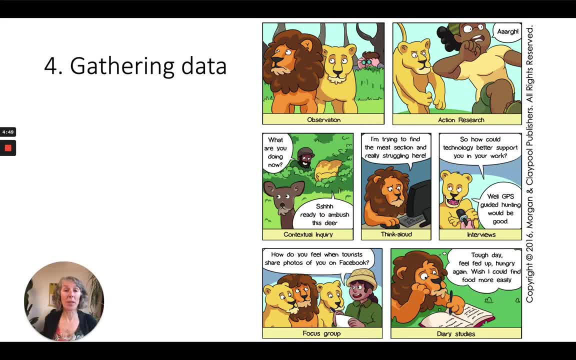 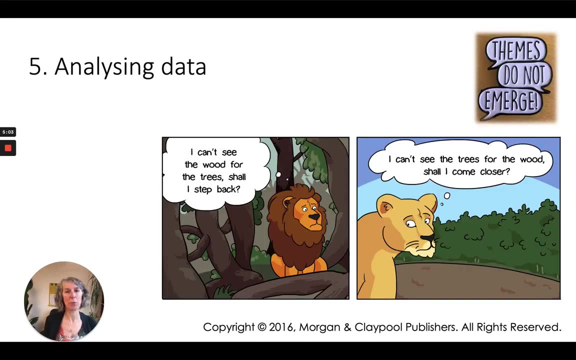 Of course, these techniques may often be applied in combination or adapted, for example, for much more online data gathering. But we go through those seven in detail on the assumption that once you've mastered those seven, then you have a good basis on which to adapt, from which to adapt. 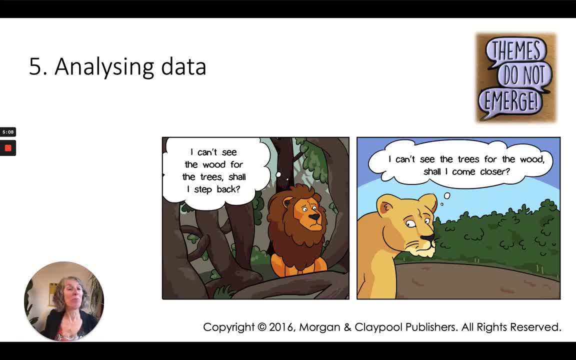 In terms of analysis, we think about different qualitative methods, But essentially there's an iteration between really analysing the data, getting to grips with the data and stepping back and seeing the bigger picture. As much My extra little photo in the top right hand corner here reminds us. you know, themes don't emerge. 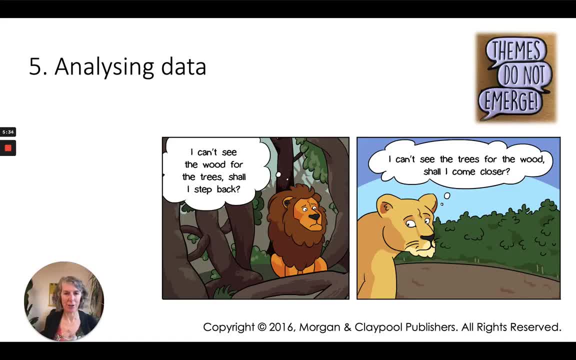 You, as a researcher, identify themes. You bring your own understanding, your own interest, your own interpretation to the data. So in analysis it's important to be reflexive about how you go through that iterative process of constructing narrative, checking against data, being driven by the data. 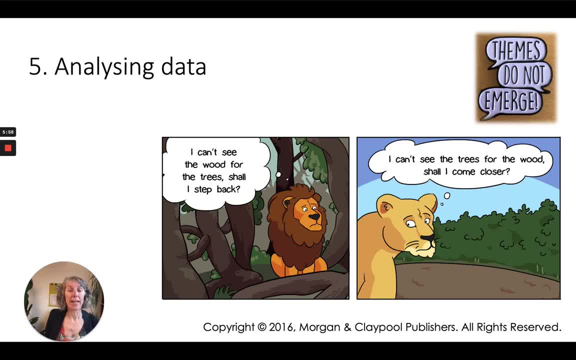 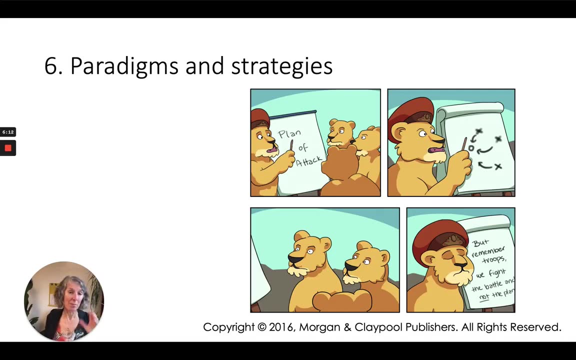 In order to develop a good narrative that is faithful to the data at the end of the day and also interesting and important. As I kind of already hinted, you very often don't just apply one method. You will often apply multiple methods and construct an overall process around multiple methods of data gathering and even possibly, multiple methods of analysis. 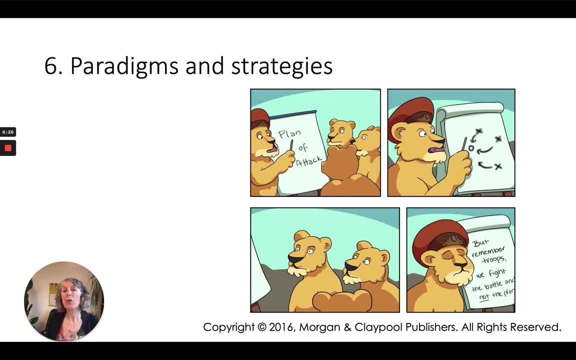 So the components of a qualitative study can be put together in different ways, And there isn't one way that is right to the exclusion of all others. For example, grounded theory explicitly interleaves data gathering and analysis, whereas most approaches to thematic analysis presuppose that the data has been gathered already. 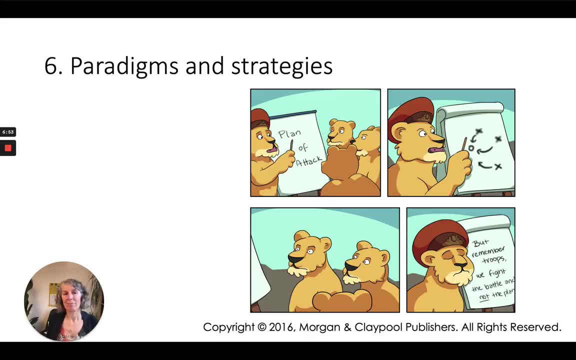 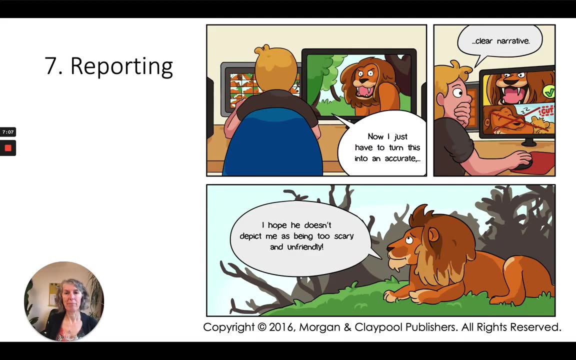 Neither is right. Neither is right and all others wrong. What matters is that the approach suits you as a researcher, suits the research question and is also appropriate to the situation. Often, the final step is the reporting of results, And it's really important to balance clarity of findings. 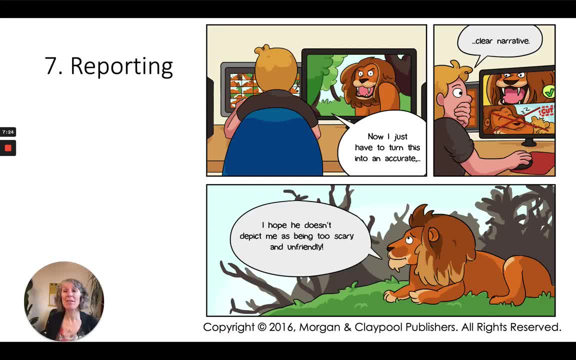 So that the narrative can be understood by others with an honesty that means that you're not producing a biased account, And it can be challenging to achieve this balance between honesty and clarity, So we discuss issues around how you report and how you build the narrative. 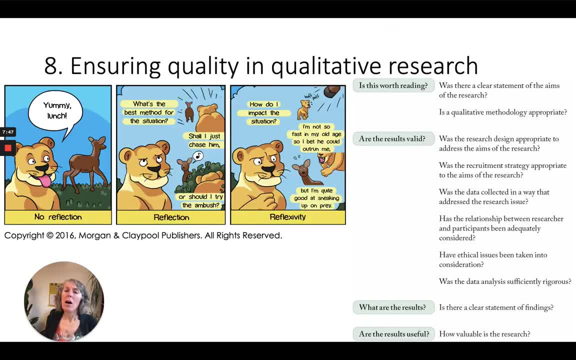 One of the challenges with qualitative research is that it can often be regarded as kind of wishy-washy and vague and unreliable. So we discuss explicitly how to maximise the quality of your study. There are lists of qualities of qualitative research, such as you know. actually, is it worth reading?